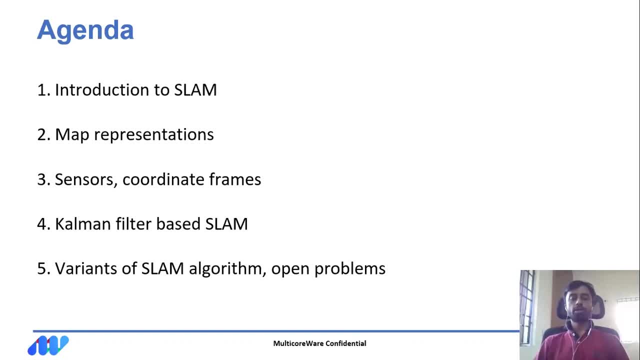 is referred to as a Kalman filter-based SLAM is explained. This is a good conceptual starting point to understand any variant of a SLAM algorithm. Finally, we conclude with the mention of different variants of SLAM algorithms and some of the open problems in SLAM research. 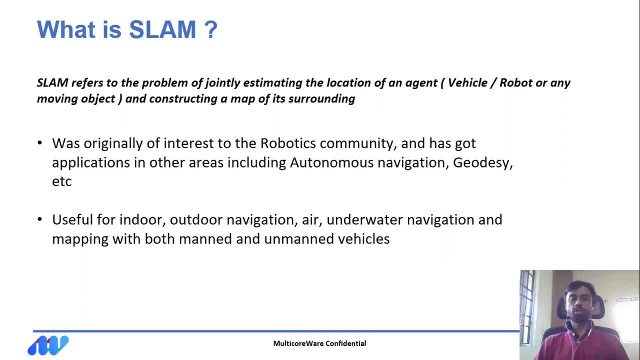 What is SLAM? SLAM refers to the problem of jointly estimating the location of an agent. An agent could be a vehicle, robo or any moving object and also construct a map of its surrounding. We assume that we have an agent which moves in a region. and we find a slope of 8-1-1, and we can simulate that argue. we find a slope of 8-1-1, and we can facilitate that argue. We can also calculate the vacancy of the slamer. We can also calculate the vacancy of the slamer. This is a running in-품。. We can also simulate theестeralie of a slamer. So the ending of SLAM is that which göbe 1 km per minute. What is SLAM? Shall we look into all of these? 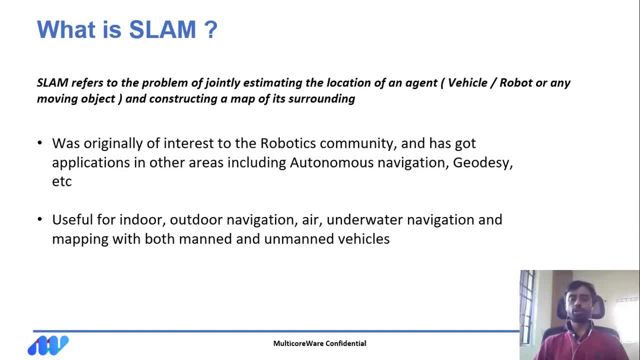 Please do this to determine our problem of LOCKD, would like to estimate the location, the precise location of the agent, and we want to know what exactly is the surrounding, which means, uh, what are the obstacles in the surroundings and what, what are the positions of these obstacles? so this problem was of interest originally to 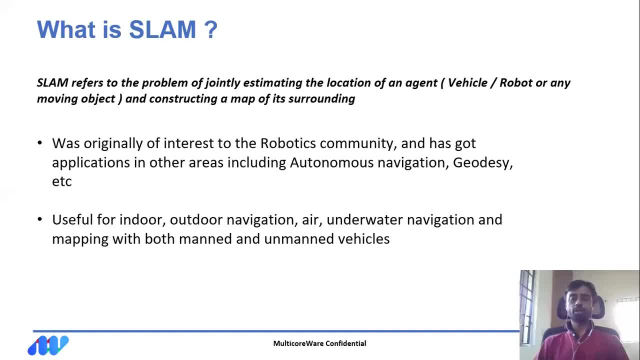 the robotics community and it has got applications in various other areas, which includes autonomous navigation, which is which will be our focus of stock and geodesy, etc. slam is useful for both indoor and outdoor navigation, air, underwater navigation and mapping in both unmanned and manned vehicles. so here is an illustration of the slam. 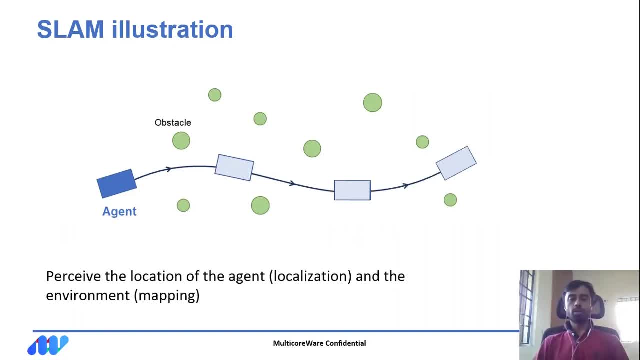 problem. we have an agent that is being shown in this figure as a blue rectangle, and you can also see the trajectory of this agent, which is the path along which the agent moves. and along with this path, various positions taken by this agent at different points of time are shown as rectangles. 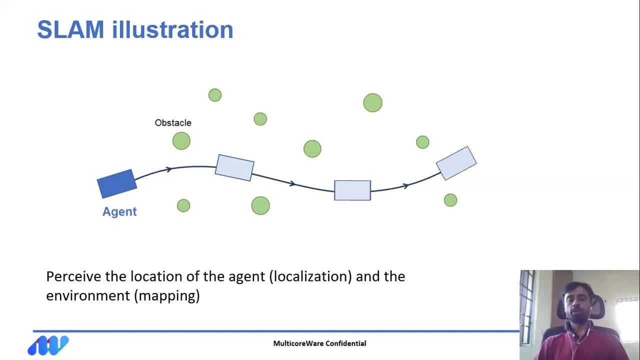 we can also see a plot of some of the obstacles in the region where the agent would navigate. these obstacles are shown as green circles here. in general, these obstacles could be of varying sizes and shapes. we would like to perceive the location of the agent at different points of time. 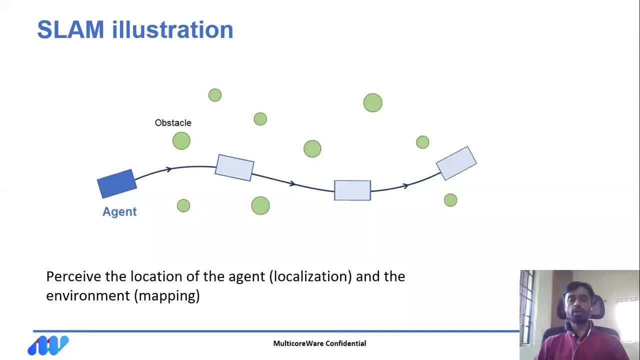 which is referred to as localization, and also perceive the location of the obstacles in the region of navigation, which is referred to as mapping. here we assume that these location obstacles are static, which means they don't move and they hold the same position at any point of time. 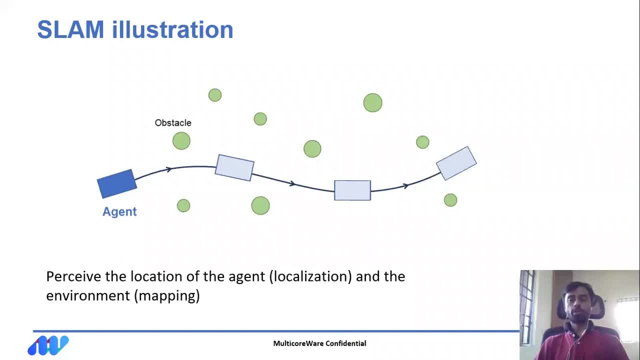 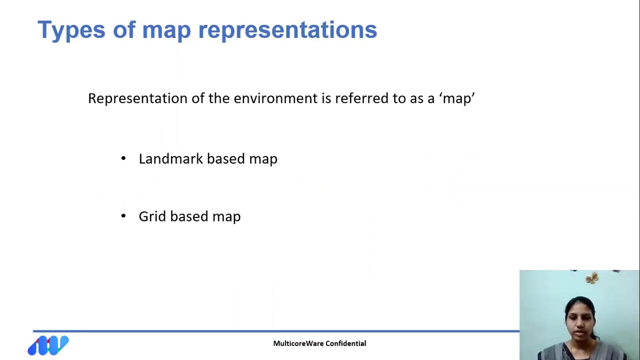 the next few slides will be taken over and taken over by my colleague, trisha rachet. map is a representation of the environment in which the agent travels. map contains the information about the obstacles that are surrounding the agent. there are two ways to represent a map. 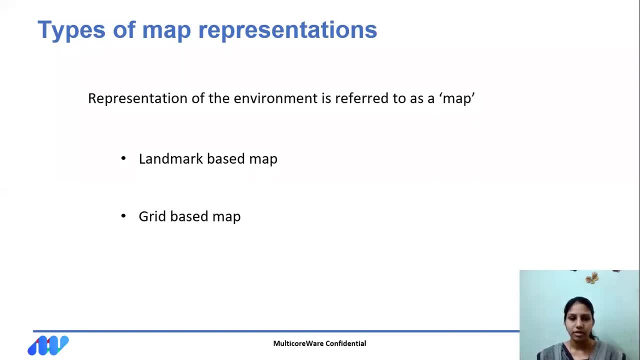 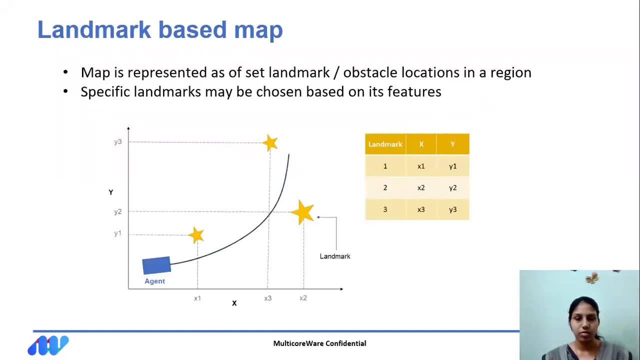 one is the landmark based map and another one is the grid based map. landmarks are stationary objects in the area environment which can be distinguished easily and re-observed. When the agent travels through the environment, it observes many obstacles, of which only some are classified as landmarks. A landmark-based map. 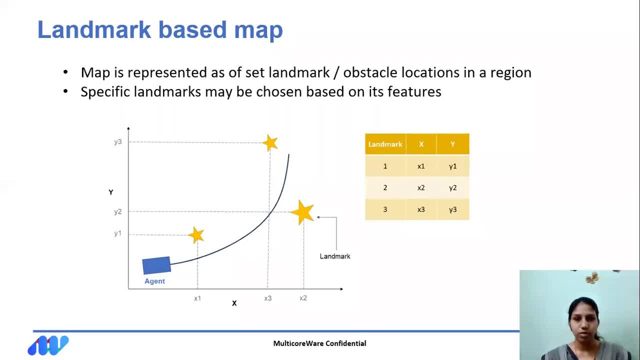 contains the set of locations of the landmarks which were observed over a time. In the figure we can see the stars represent the landmarks and the agent moves through a trajectory. It observes the landmarks one by one while moving. It also estimates the position of the landmarks. 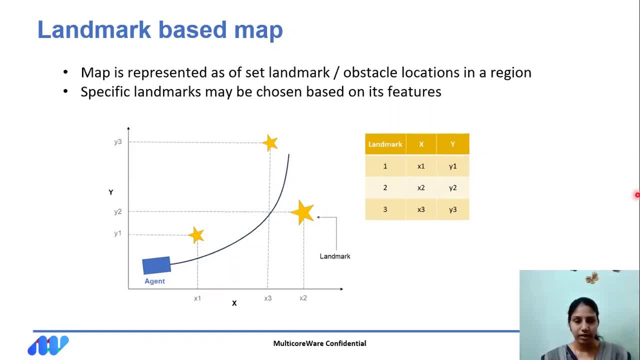 The first landmark has position coordinates of x1 and y1.. Similarly, the other landmark's position will also be estimated and recorded. This is termed as the landmark-based map. We can also see the position coordinates of the landmarks are listed and maintained as a table. 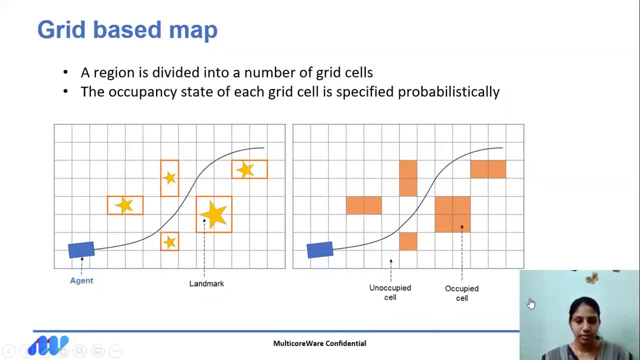 Another type of map representation is a grid-based map. As the name says, in a grid-based map, the region is divided into a number of equally spaced grid cells. Each grid cell can have an occupancy state of either occupied or unoccupied. When a cell is termed to be an unoccupied cell, 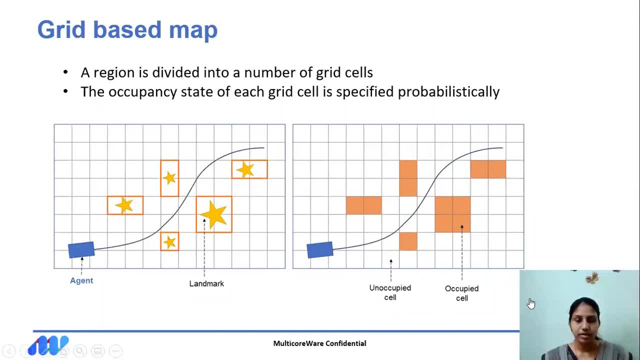 it is free from any obstacle. When a cell is termed as an occupied cell, it indicates that the region has some obstacle. In the figure towards the left we can see stars which represent the landmarks and an agent which is traveling through the environment. 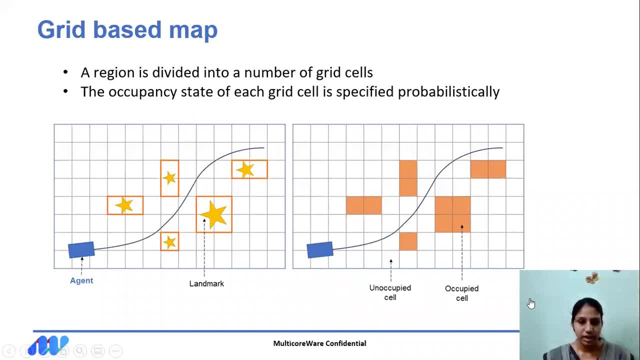 We want to estimate the state of each of the grid cell probabilistically. When the occupancy state of the grid cell is the occupancy probability of the grid cell exceeds a certain threshold, the cell is marked as an occupied cell. Similarly, for all cells, the occupancy 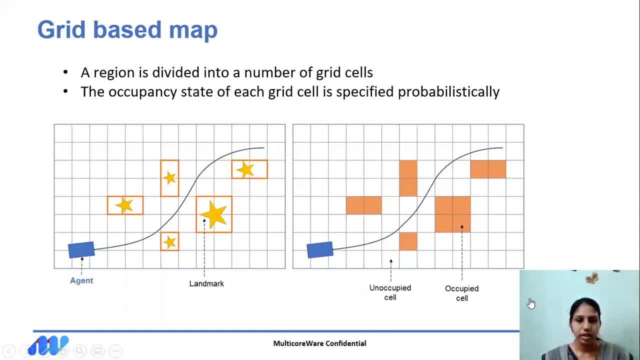 state is estimated In the figure towards the right. we can see that the cells which are containing the landmarks are shaded and marked as an occupied cell. We can notice that even though only some region of the cell has the landmark, the entire cell will be marked as an occupied cell. 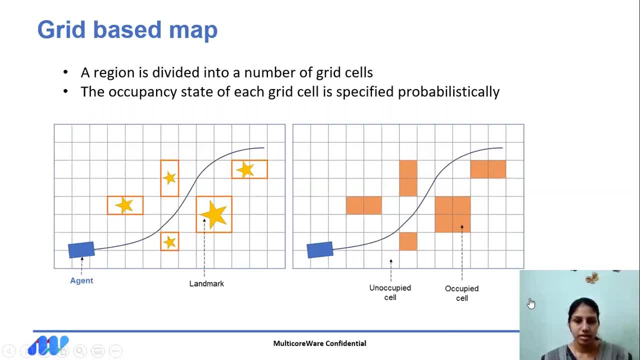 This is because the occupancy state can only have two values: which is occupied or unoccupied. In real life scenario, there is more possibility that the cell's neighborhood to the occupied cell will also be marked as an occupied cell. But here we don't make that assumption. In a grid-based map, each cell has an. 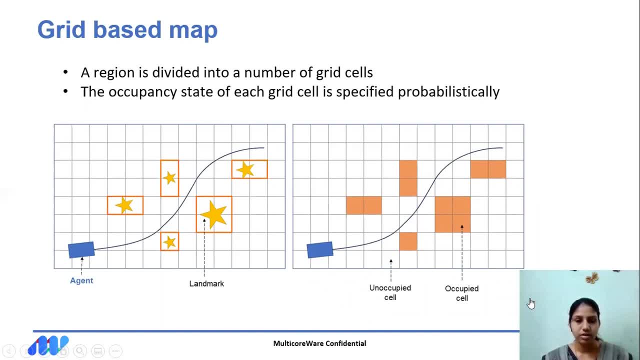 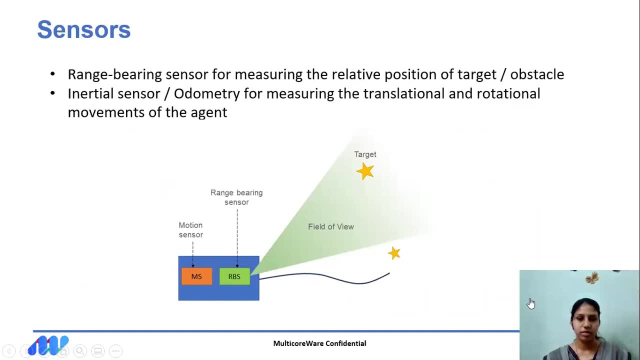 occupancy state, which is independent of the other cells. Sensors provide the measurement, which is input to the SLAM algorithm. SLAM makes use of a range-bearing sensor and a motion sensor. Both of them are mounted on the grid. The range-bearing sensor will provide the relative position of the target, which 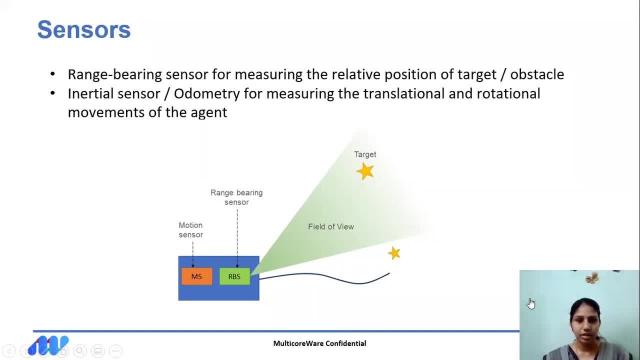 is present in the field of view. Radar, LiDAR and stereo cameras are some range-bearing sensors. Motion sensor will provide the transitional and rotational movements of the agent. We can estimate the position and orientation of the agent relative to its starting point. 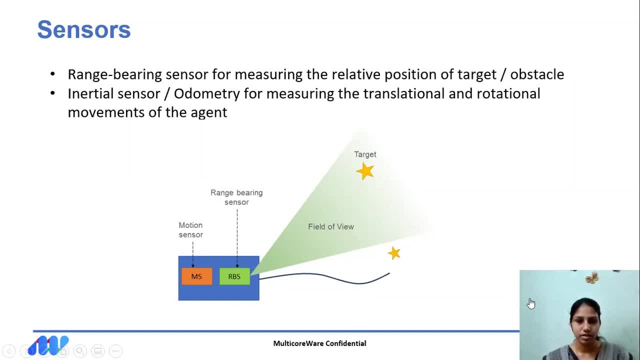 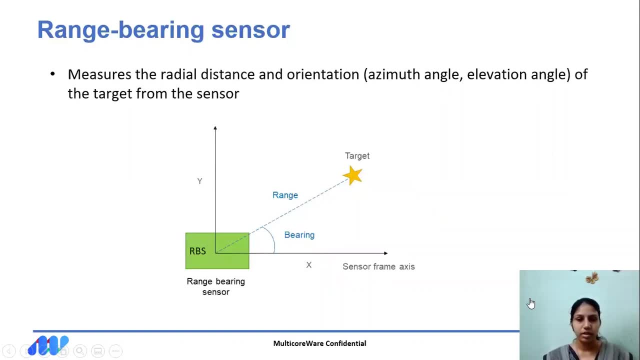 Inertial sensors and odometry are some motion sensors used. Range-bearing sensor will provide us the relative range of the target with respect to the sensor. It also provides us bearing angle, which is azimuth, and elevation. Azimuth provides information about the direction in which the target is present. Elevation angle provides information about. 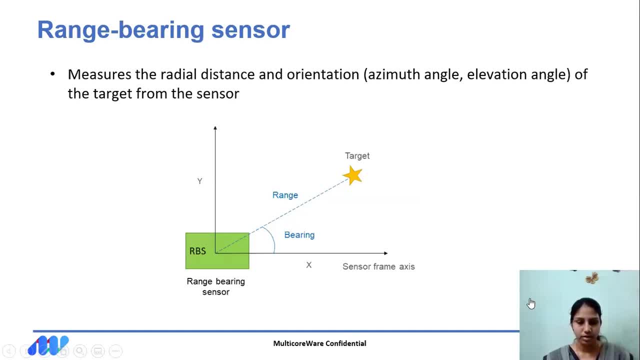 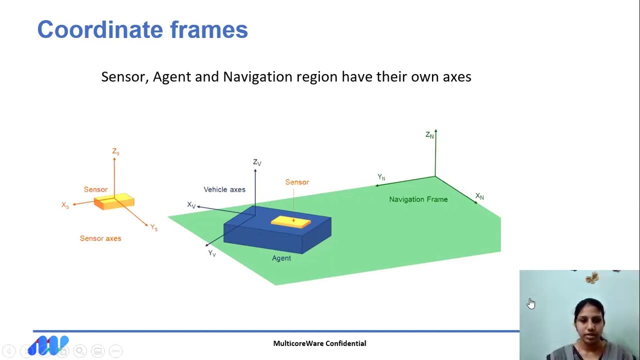 how high the target is placed with respect to the sensor. All the measurements from a sensor is in the sensor frame axis. Sensor provides us the measurement in sensor axis. It is represented as XS, YS and ZS in the figure. The sensor will be mounted on an agent or a vehicle. The agent has its own axis, termed as the. 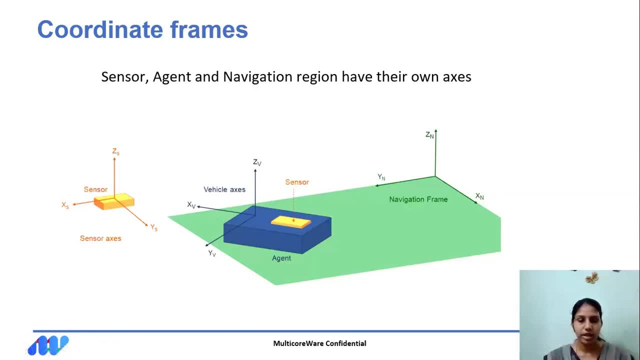 XV, YV and ZV. The agent will move around the region and hence the vehicle axis will keep changing. Thus it is necessary to have a common frame of reference to mark the locations of the landmarks and the agent. This is known as the navigation frame. The region in which the agent travels is 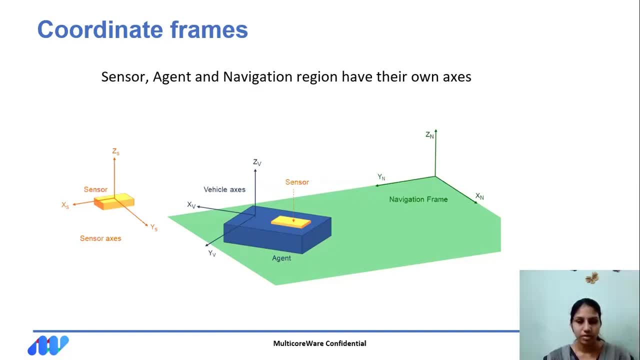 the navigation frame and the navigation axis is present in the starting point of the agent. It is the stationary and hence it is useful to mark the locations of the landmark as well as the agent. Now I request my colleague Karthik to take over the next few slides. 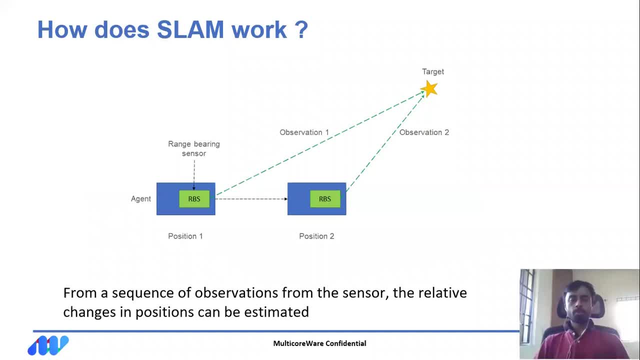 In this slide. it illustrates how SLAM works on a top level, And this is the underlying principle on which SLAM works, irrespective of which variant of SLAM algorithm we use. In this figure, we have shown the positions of the agent at two different points of time. 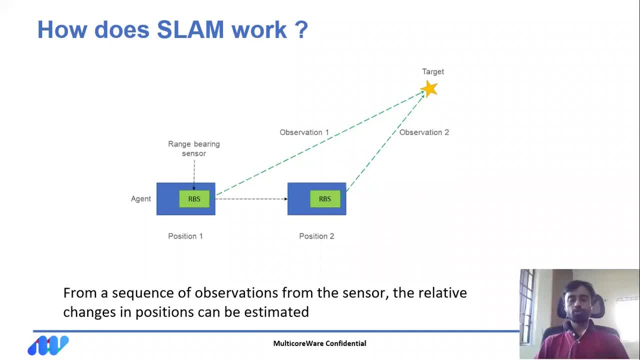 mu, position one and position two, And you can see that the agent also mounts a range bearing sensor. We have shown the landmark as a green star. We have just shown one landmark for illustrative purposes. The range bearing sensor takes measurements of this landmark. 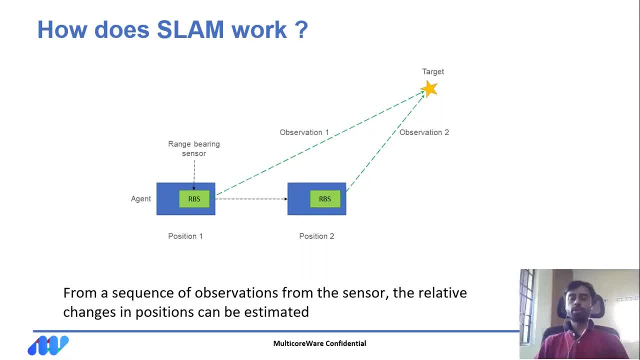 from these two different positions. The first measurement is labeled as observation one and the second measurement is labeled as observation two. Now we see that observation two is different from observation one because position two is different from position one From the change of observation from observation one to two. 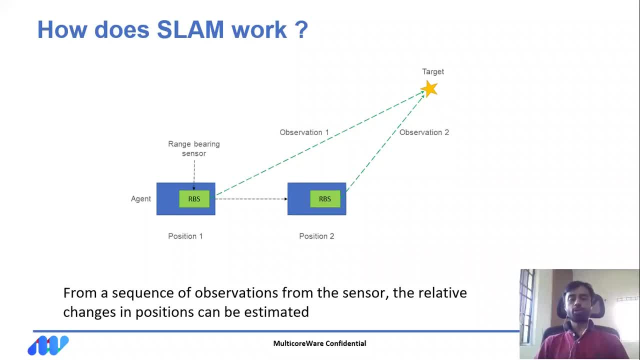 we can infer the change of the relative change of position two. So we can take an example of the same thing from position one to two. We can geometrically calculate this. In general, we can say that when we take a sequence of observations, then from the sequence of observations 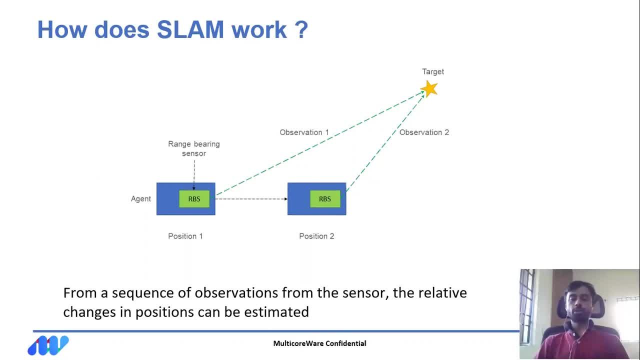 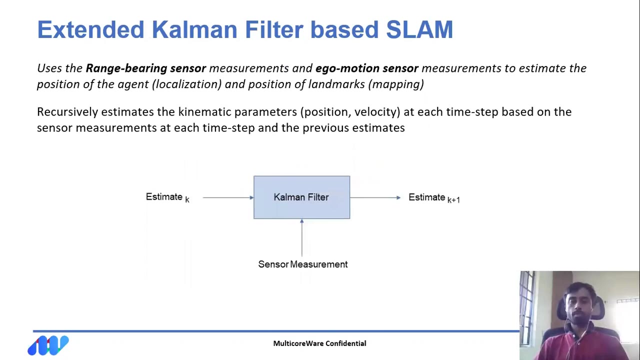 we can infer the relative changes in position of the agent. So this is an underlying principle based on which SLAM works. so now we move on to uh, what is meant by extended kalman filter based slam? this is one variant of slam algorithm and it's also a good conceptual starting point to understand. 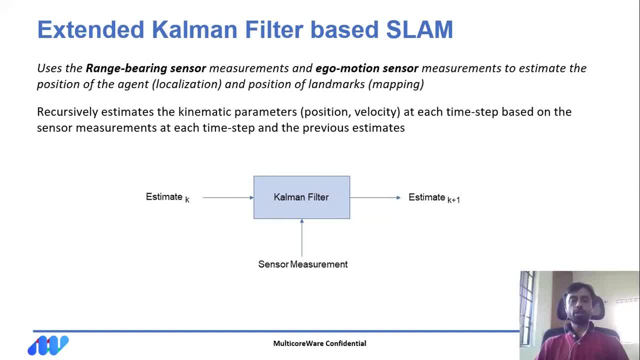 any variant of slam algorithm because many of the ideas here are carried over to other variants of slam algorithm. the common filter based slam uses a range bearing sensor and also an ego motion sensor optionally to estimate the position of the agent and the position of the landmarks. we can see a figure variant we have. 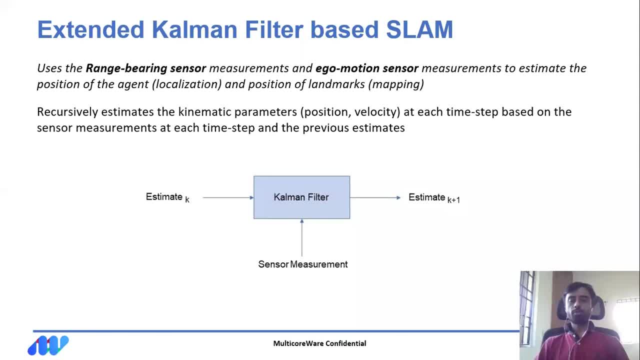 plotted. we have shown the kalman filter as a block. it takes us input the estimate of these parameters which we in which we are interested in, and it includes the position of the agent and position of the landmarks and optionally we could have the velocity and acceleration of the. 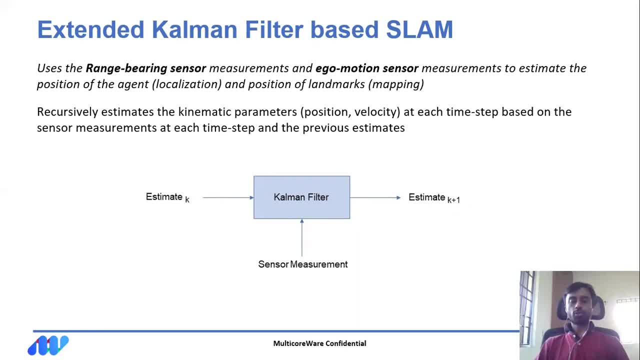 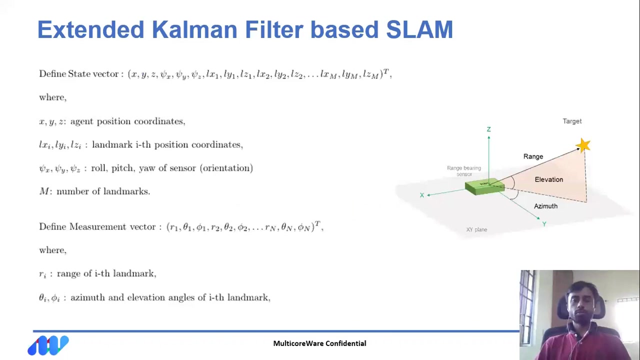 agent as well. it gives the estimate uh, it takes us input the estimated time, step k. and also it takes us input the sensor measurements and it gives us output the estimate at time, step k plus one. before we move on to an explanation about how the extended kalman filter. 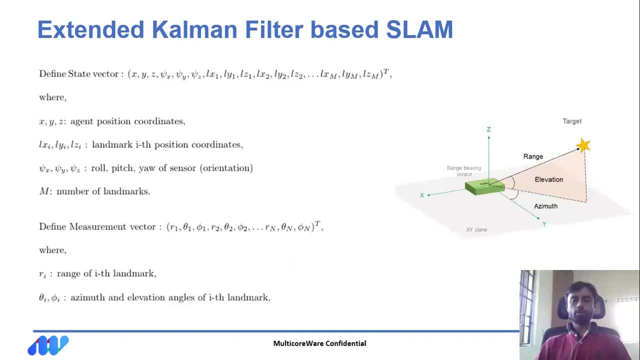 based slam works. let's define some of the parameters with respect to the extended kalman filter based slam formally. firstly, we define what is meant by the state vector. The state vector comprises of the components x, y, z, which are the agents, position coordinates, lx1, ly1, lz1, through lxm, lym, lzm, which are the landmark position. 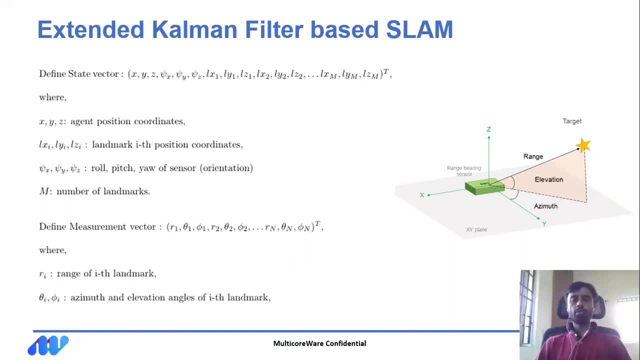 coordinates. Here, m is the number of landmarks we have. We have the orientation in terms of roll pitch and yaw, denoted by phi x, phi y and phi z. We define what is the measurement, what is referred to as a measurement vector? 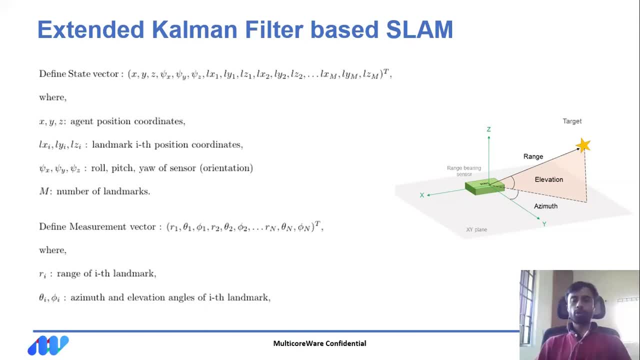 This comprises of the components r1, theta1, phi1, through rn, phi n, theta n. Here r1 is the range of the i-th landmark, which means which is the distance, the radial distance of the landmark from the center. This is the center of the axis of the sensor And theta1 and phi1 represent the elevation and azimuth. 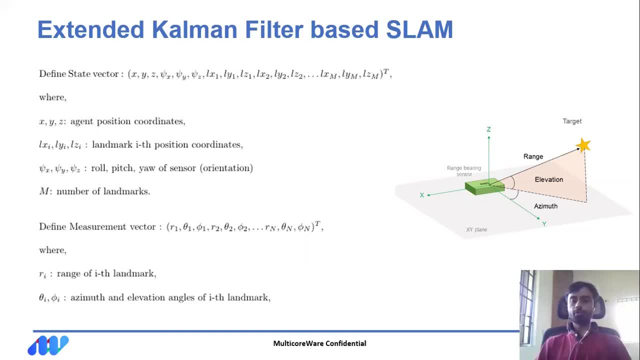 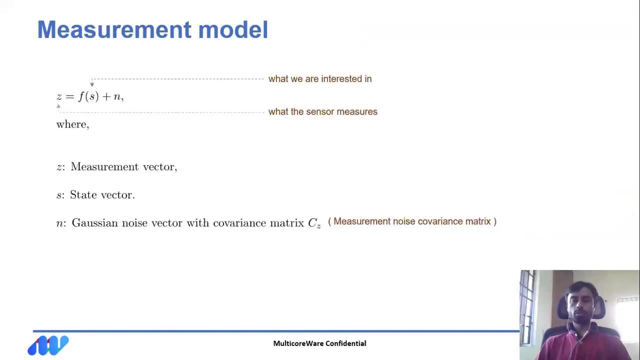 angles of the landmark with respect to the sensor axis. We can see a plot of the range, elevation and azimuth in the figure shown in the right hand side. Let us define what is meant by measurement model. A measurement model is a mathematical model for what the sensor measures. The measurement 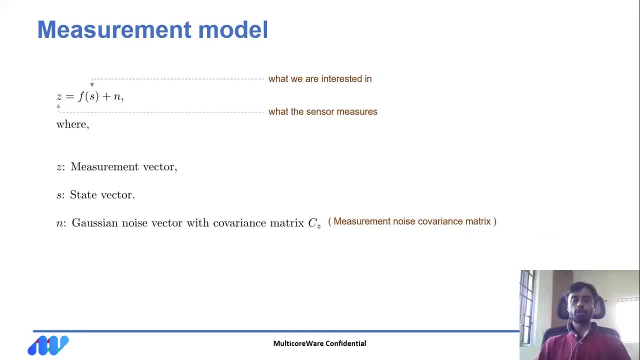 z is equal to f of s, which is some function of the state vector plus some Gaussian noise n. The measurement vector is what the sensor measures and the state vector is what we are interested to compute, estimate. We see that the measurement vector is some function which. 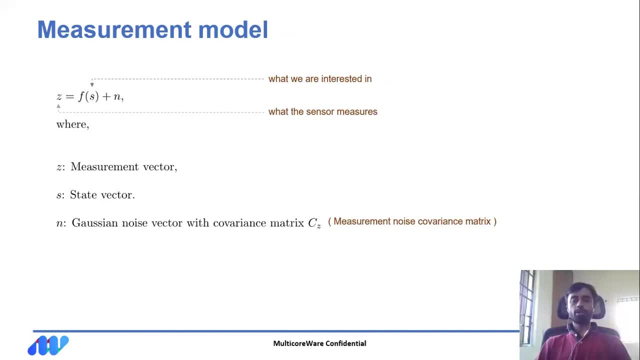 could be a linear or non-linear function, and it is also corrupted by some Gaussian noise which is random in nature. We assume that the Gaussian noise vector has a covariance matrix represented by C e z. This covariance matrix is often referred to as the measurement noise covariance matrix. It models the uncertainty in the sensor measurements, or in other words, 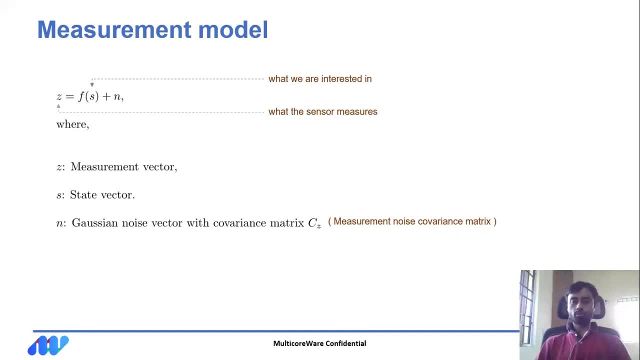 the sensor noise. Let us define what is then called as a state transition model S of k plus 1, which is the state at time step k plus 1 is equal to some function of state at time step k plus Gaussian noise at time step k. 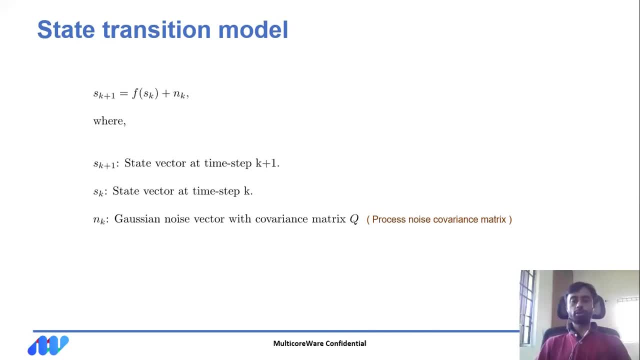 This model models the way the state parameters change over time. In general, the position of the agent, the velocity of the agent and also the orientation of the agent can change with time because the agent is moving and therefore we have a model for how the state 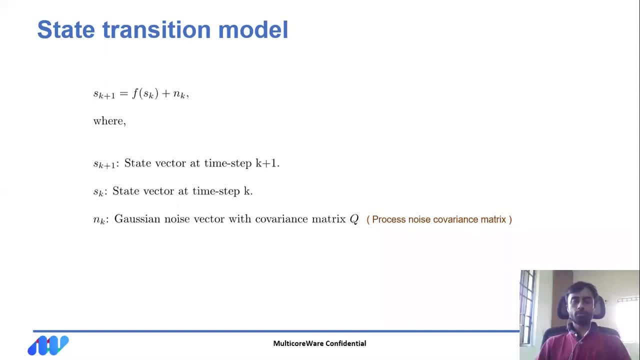 changes, state parameters changes And we also have a noise here because there is some underlying uncertainty in the way the state changes. The noise vector here has a covariance matrix which is reannoted by q, and this noise matrix is often referred to as the process noise covariance With regard to the Kalman filter. 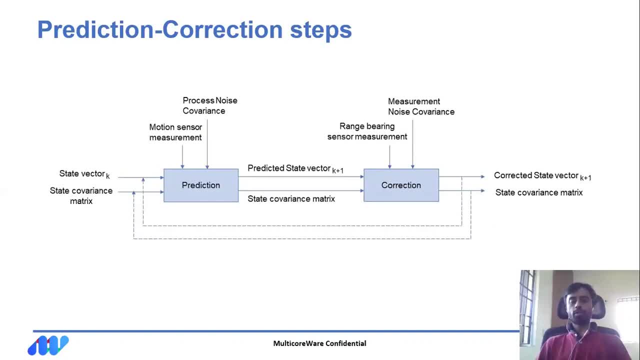 external Kalman filter. we have 2-D-D-Celta- Okay. Okay, two main steps which are referred to as the prediction and correction. we can see in the figure that we have one block which shows the prediction and another block which shows the correction step. 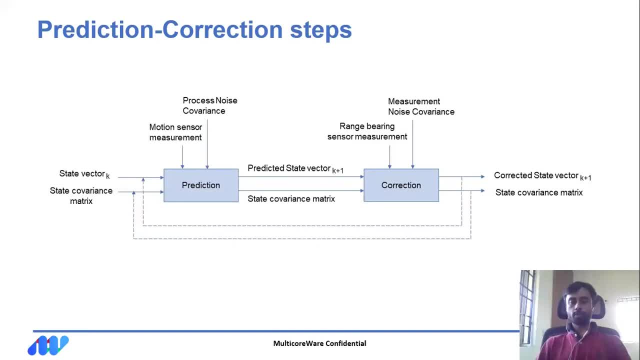 let's focus on the prediction step first. the prediction step takes as input the state vector at time, step k- and also the covariance matrix, which is referred to as the state covariance matrix. the state covariance matrix models the uncertainty in the state at time. step k: the prediction also takes this input, this measurement. 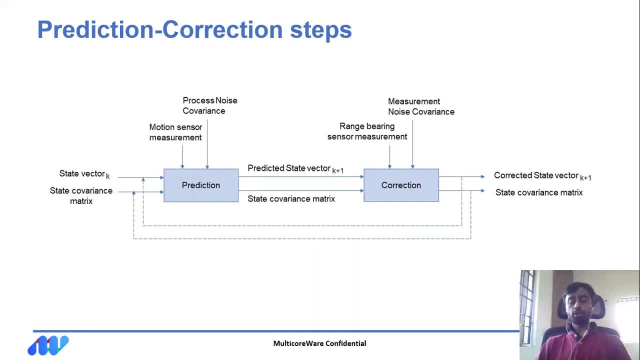 as the measurement from the motion noise motion sensor and its corresponding process, noise covariance, which models the uh noise in the sensor. the prediction step gives an output of the predicted state at time step k plus one using the state vector at time step k, and it also gives the state covariance matrix. 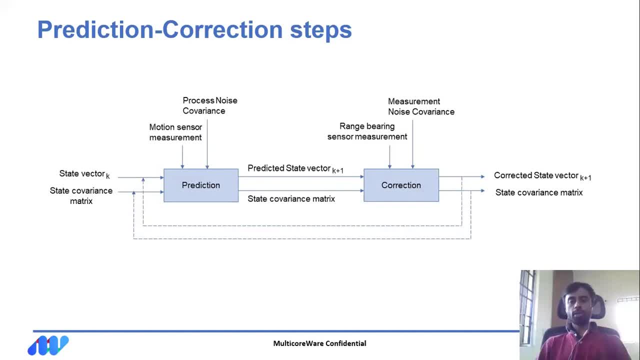 the predicted state vector is computed from the state vector at time, step k, using the model for the covariance matrix process transition which we defined in the earlier step, or the state transition model. so, basically, we used a state vector at time, step k and predict as to how this state vector 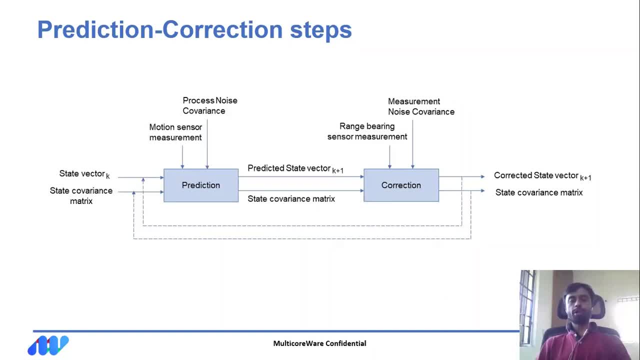 could have changed to a timestamp k plus one. we predict the motion of this motion of the wake agent and we predict how, in regard. in this regard, we predict how the uh position of the agent, the velocity and acceleration would have changed, sometimes from k to time step k. 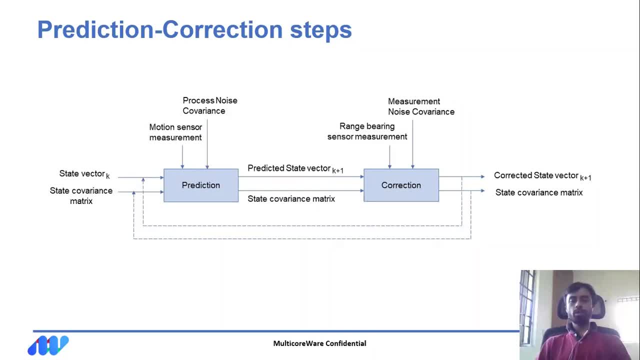 step k plus one, and the uncertainty in this prediction is modeled by the state covariance matrix. the correction step takes this input: the predicted state vector at time, step k plus one, and also the state covariance matrix which was computed, which which are computed from the prediction block. the correction step computes the corrected state vector. 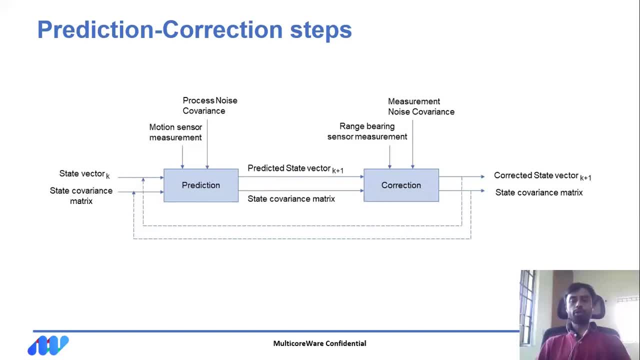 at time, step k plus one and the corresponding state covariance matrix for this. the correction step uses the range bearing sensor measurement, which could be a radar or a lidar or some other sensor, and it also uses input of the measurement, noise covariance matrix, which models the uncertainty. 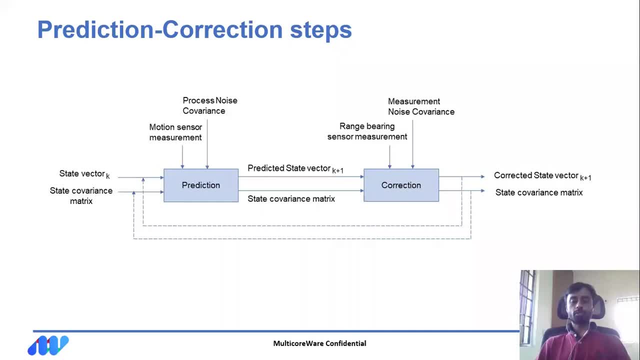 or the noise in the range bearing sensor measurement. while the prediction step predicts the state vector at time, step k plus one using a mathematical model, the correction step uses the sensor measurements to compute where exactly this vehicle was. it uses the range bearing sensor measurements to correct the error in the predicted. 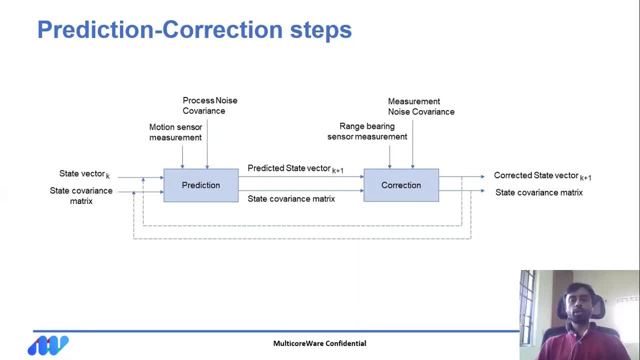 state vector and it also computes the landmark positions using the measurements from the range bearing sensor machine. now the corrective state vector at time step k plus one is again fed back to the prediction step input for the next iteration. so this, these prediction correction steps, operate on a recursive manner to at every iteration. 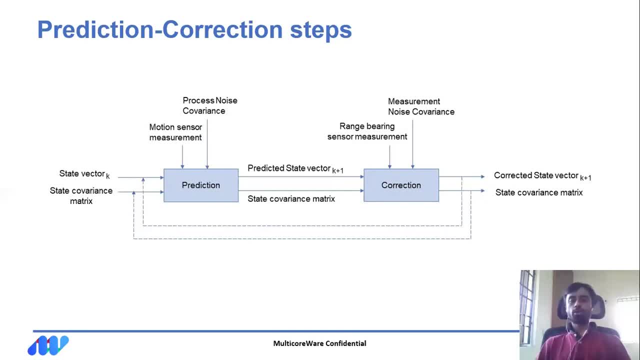 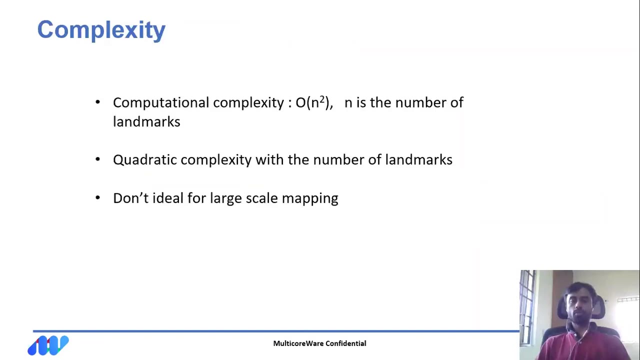 taking the input of the sensor measurements to compute the state vector at that point of time. with regard to the complexity of the computational complexity of the kalman filter, it's in the comment filter. it is in the order of n square where n is less same than the xn of h noise along n workings and n power. with respect, this can also be computed as the polygonal field of the aim can also mind aim measurement motion with respect to the mesh system. and that is also until we are working with analysis in the device as we is learning the vector, faishtool or preventative, those fixed terms of edge engineering problem rivals are of kleinstein vs pascal poorос. the perfect technique. you have to increase the probability that there are other relationships in the stage vector, taking the input of the sensor measurements to compute the state vector at that point of time. 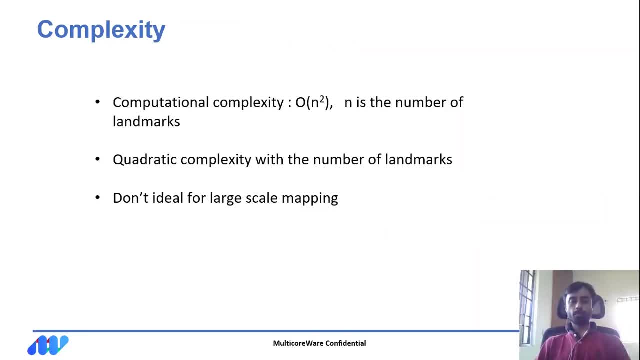 the number of landmarks. we see that the computations required for uh extended complement filter is not is quadratic with respect to the number of landmarks n, which means that as n increases, that is the number of landmarks. when the number of landmarks is large, the computations required become very large. 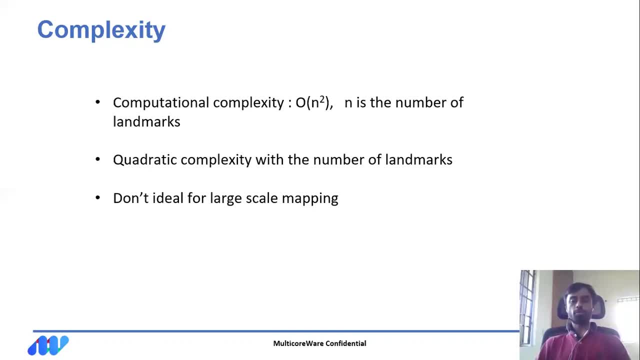 therefore, when we have a large scale mapping problem, wherein we have a large map with a number, many landmarks, a large number of landmarks, then using an external component filter based lamp would imply high computation complexity and it becomes infeasible. so we see that using the external component filter baseline or ekf. 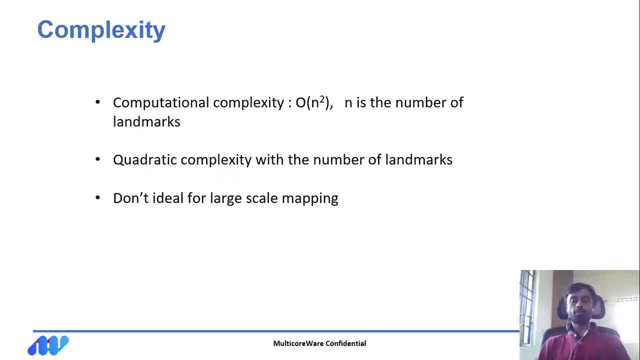 is not ideal for large scale mapping. however, we can use it for very small scale mapping wherein we have a very small number of landmarks. here is the list of the methods we have for different methods. we have, for example, an external student filament system which we can consider in this virtual reality. 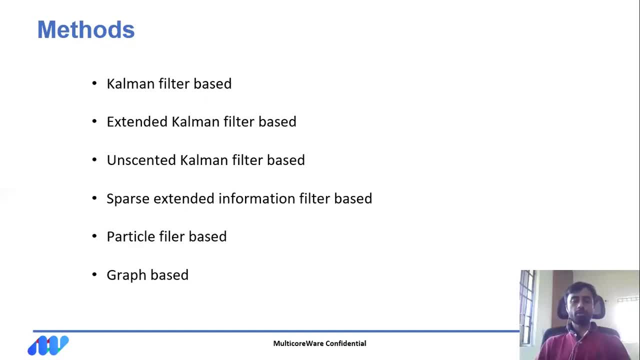 but keep in mind that we are using the external component filter based sun. we have the external component filter based slam, we have the comment filter based lamp, we have the extent of common factor based lamp, we have the unscented common filter based lamp. so, within common filter based family of slam itself, we have 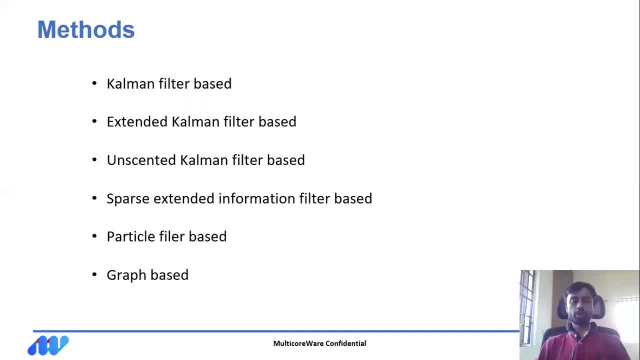 at least three varieties of three variants. so what we looked into is specifically the external carbon filter based lamp, standard information filter based SLAM. We have the particle filter based SLAM and finally we have the graph based variants of SLAM. We see that, while we have a number of methods available, 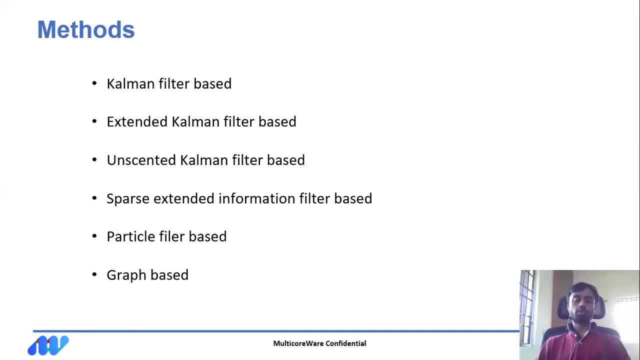 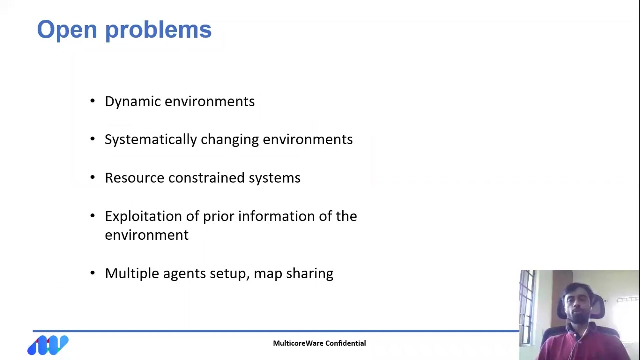 each of them have its own pros and cons. With regard to the computation complexity and the flexibility of the SLAM algorithm, it varies from one algorithm to another. in this list, Here's a list of some of the open problems in SLAM research. 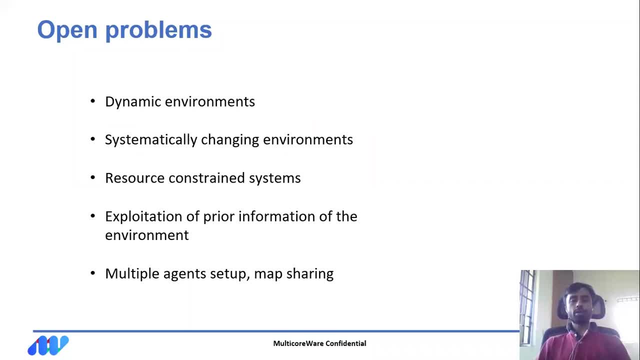 I told that we we assumed that the environment in which the agent navigates is static, which means that the obstacles are assumed to be in static position. However, in real life scenario, it's very rare that we have the obstacles being absolutely static. 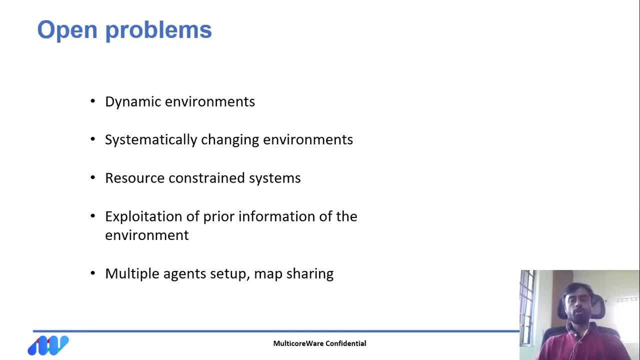 At least in on-road scenarios. So it remains a challenge as to how to adapt SLAM to dynamic environments wherein the obstacles could change, change position over time. a related problem is what is referred to as systematically changing environment variant. the obstacles do not change very. 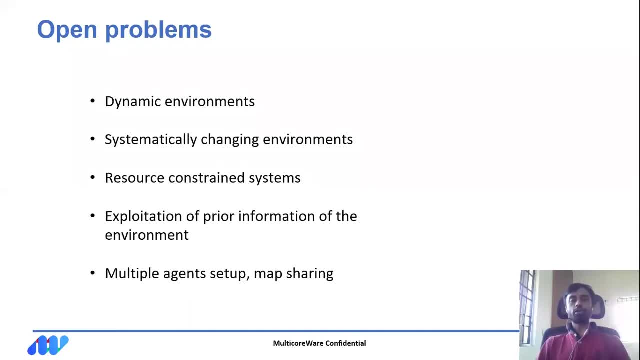 rapidly. however, it undergoes a change in systematic manner. for example, let's take a bad horse environment or industry set of current. the exact placement of obstacles in the region where this agent navigates is known by us and at a certain point of time, we know that the obstacles could be placed in a certain 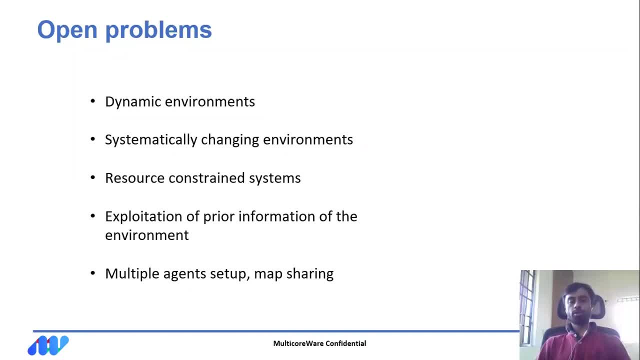 way and another point of time we would be aware of, we are aware of, we are all aware of the fact that obstacles could be having a different setup, so this is referred to as a systematically changing environment, and adapting slam to a systematically changing environment is of practical relevance. 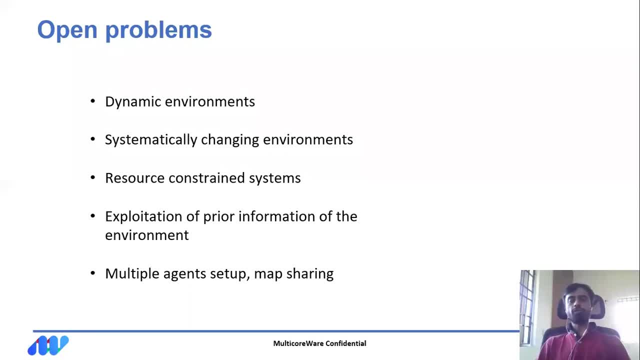 you. so we have the resource constrained systems. in most cases, when slammer to where slam is applied, we have system which is constrained in terms of the compute complexity and also the memory complexity. for example, when we have a moving robot or when we have a drone or an unmanned vehicle, the amount of 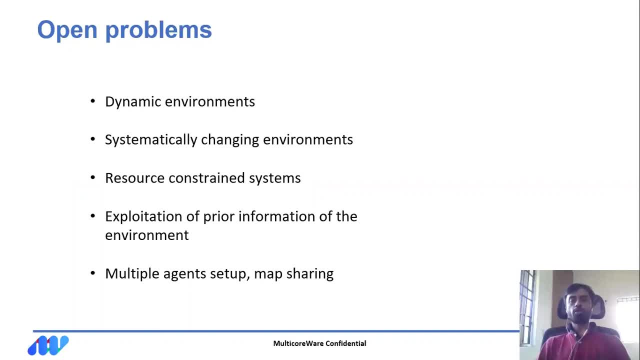 computation complexity we have and the amount of memory complexity we have is constrained. slammer, in general, is a computationally complex algorithm, irrespective of which variant we use, and adapting slam to a system which has constraints in terms of its resources is of great interest. so one of the ways this 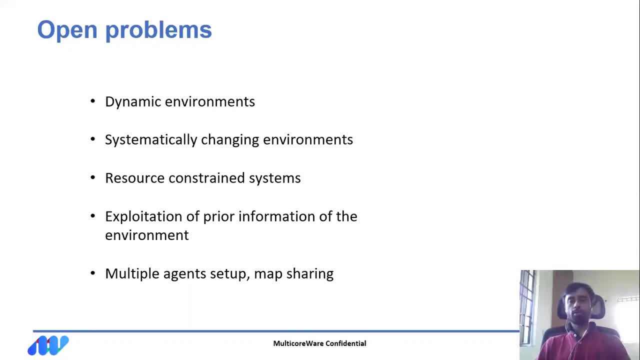 adaptation is done by not considering maps which are a global baron. we we consider maps which are local to different regions and we estimate the map, the local region variant, the agent life and finally we combine the maps to get a global map. this is one of the ways in which an adaptation to resource 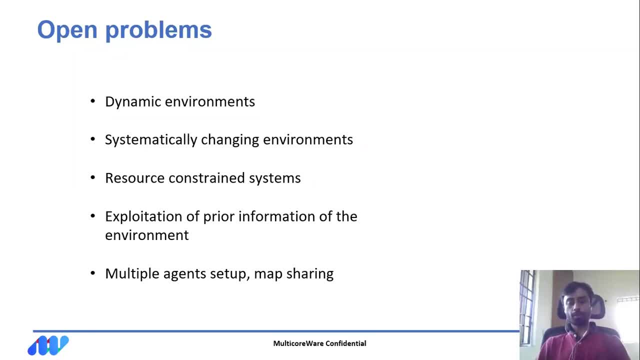 constrained systems is done, although there are other methods as well. fourthly, we have the exploitation of prior information of the environment, which means that, in case we know some, to certain extent, how exactly the map is going to be, even before we try to estimate this map, we can better, we can estimate the map more accurately. 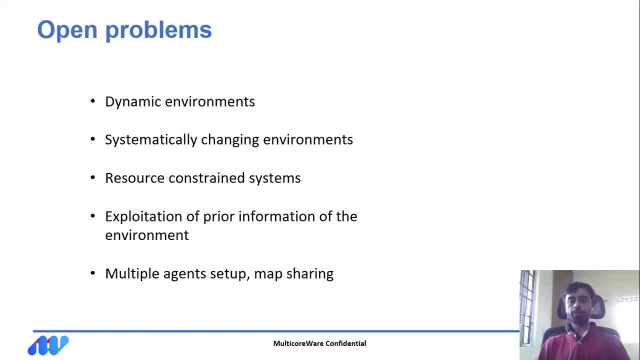 and consequently we can also estimate the agents position more accurately, because the availability of prior information, for example, in a region you might have the agent being traversing sometime ahead of the actual frame of time where you want to navigate and this could be a first-class map of being available and when the agent actually navigates this navigation. 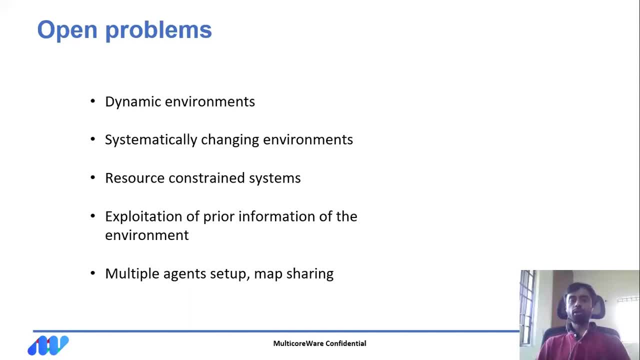 region. the map could have changed a bit. however, using a having a prior map- for instance, if you may have met a PD- would be of benefit, especially a member known or terribly powerful. how to exploring this by your map being available for the environment in which the agent navigates. it's of great. 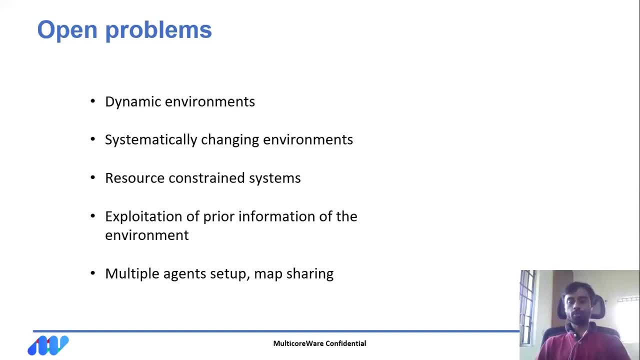 interest. lastly, we have the multiple agent shut up, set up an app sharing, which means that when we have, let's say, a cluster of agents, of cluster of robots navigating, then each agent could see a certain region of the environment in which it navigates And together the region and the maps.